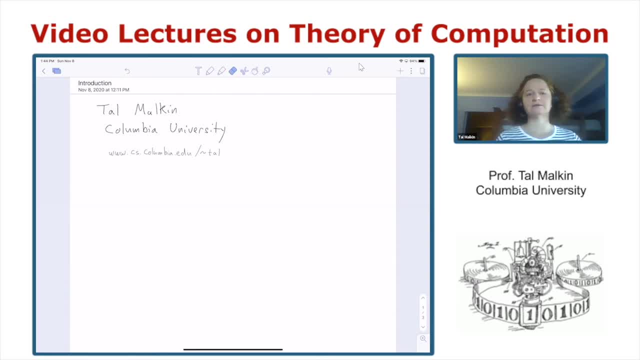 So this is an immediate connection to complexity theory, because we wanna analyze what cannot be done efficiently. There are deeper connections, there are many connections between the two of them, And in fact, defining the primitives correctly in cryptography is very important as well. Okay, so let me give a brief overview. 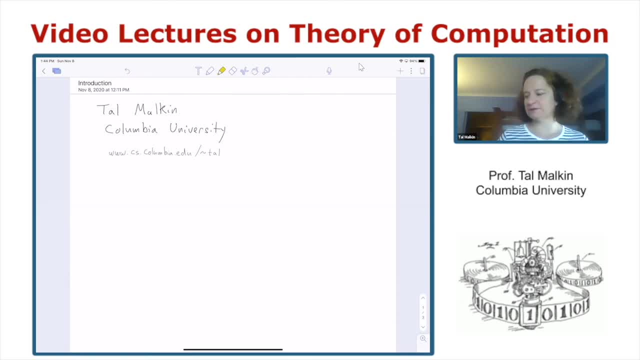 of what I will consider I'll cover in the next couple of lectures. So our topic is continuing the topic from before, which is basically about the limits of computation. It's about undecidable and or unrecognizable languages. So what you've already seen. 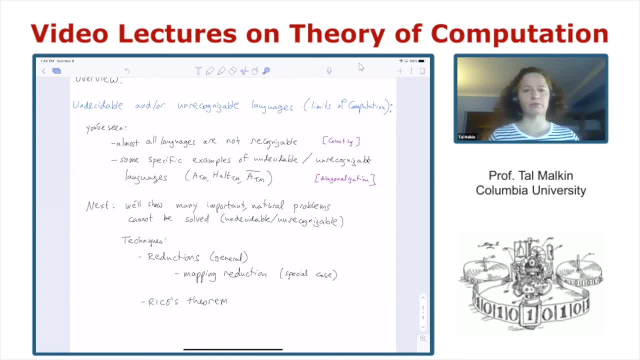 and I'll recap briefly in the beginning of the lecture. you've seen that almost all languages are in fact not Turing machine recognizable, And this can be done by a simple counting argument, And you've also seen some specific examples of languages that are undecidable or unrecognizable. 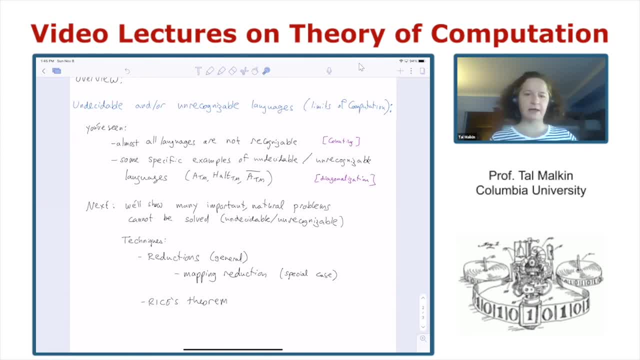 such as the halting problem, And this was done using the technique of diagonalization. Now you might think- although I would disagree, but you might think- that these examples are not very natural because it involves a program running on its own code, but it turns out to be very essential. 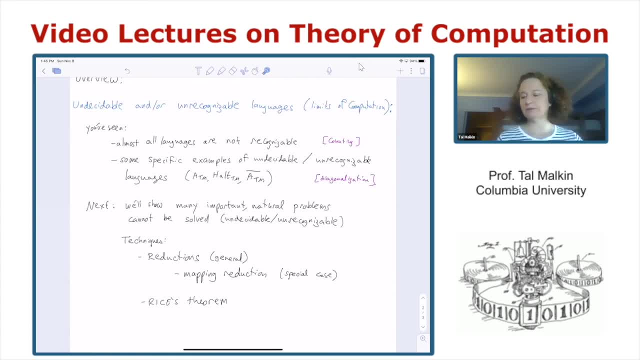 And starting from this point, we could in fact prove- and this will be my topic, we can in fact prove many, many other problems that are both important and natural, that it's obvious we would wanna solve, are in fact not solvable. 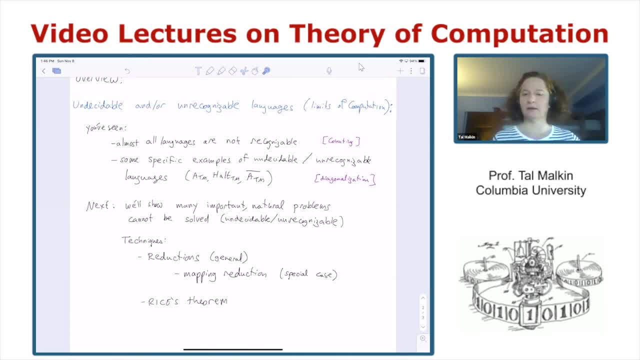 So either not decidable or not recognizable by any algorithm. Okay, so this is what we will cover. We will give several examples and general techniques. Main techniques we will cover will be reductions in general and the specific case of mapping reduction, which. 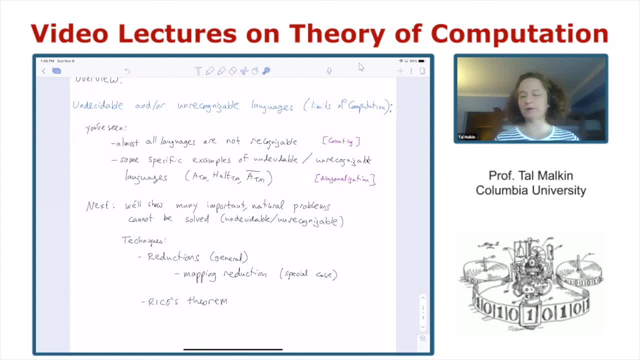 allows you to prove that some languages are not recognizable, And we'll talk about Rice's theorem, which is a very general theorem, which in some sense says that anything interesting about what a program computes in fact cannot be decided. We will talk more about that. 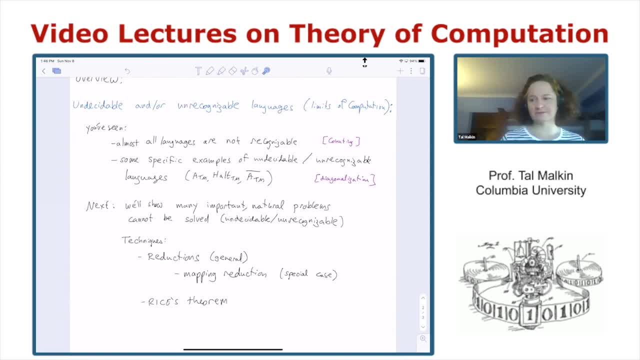 So see you in the next lectures.